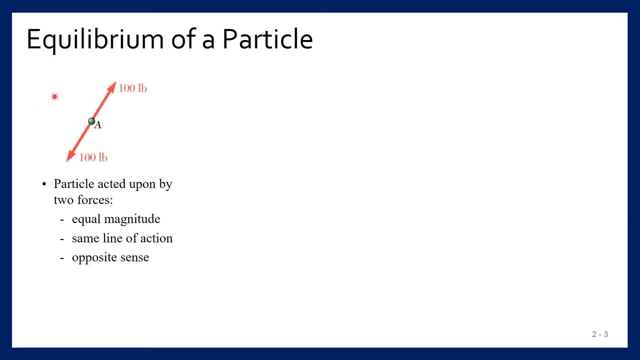 direction is opposite. So when you calculate the resultant of this, then obviously it will be zero. So we can say that this particle is in equilibrium because the resultant of the forces acting on this particle is zero. Now suppose if more than one forces are acting. 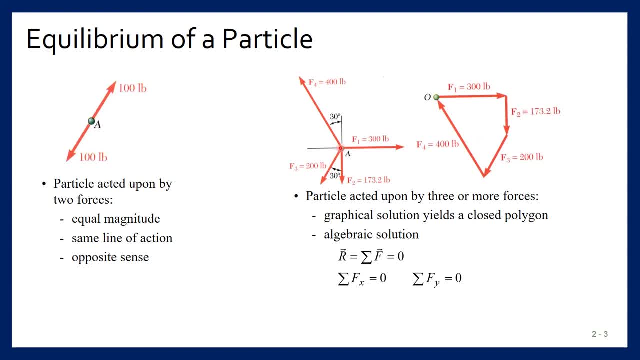 on the body. So this is the body or particle A, and there are two forces, sorry, four forces are acting: F1, F2, F3 and F4.. So now, when you calculate the resultant of these four forces, and if the resultant is zero, then this particle will be in equilibrium. 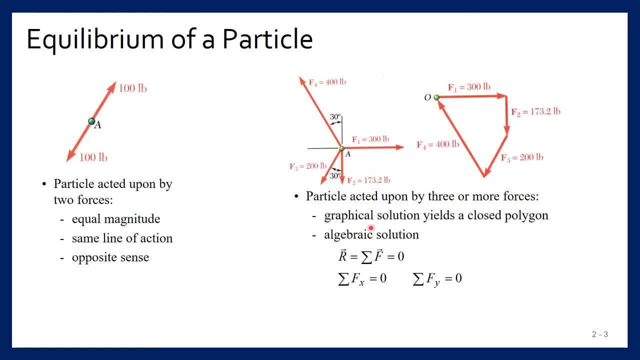 Now the resultant can be calculated by using the graphical solution. so when you will be using a graphical solution, then suppose this is the F1.. So suppose I have drawn the F1 like this, and from tip of the F1 I have drawn F2, and from tip of the F2 I have drawn 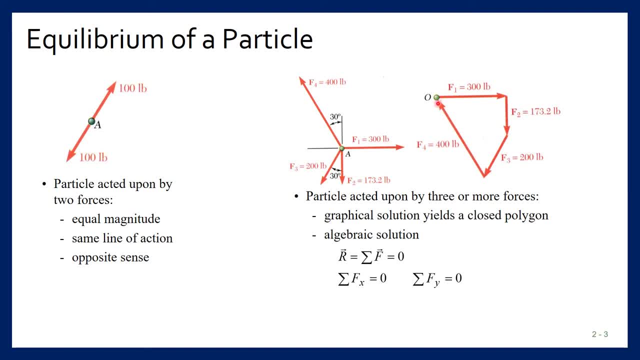 F3 like this and F4 like this. So in case of the particle in equilibrium, the resultant should be zero. that means all the forces that are acting on this particle should be, should form a closed polygon. only then the resultant will be zero. So if you use graphical method, then if you start from one force and 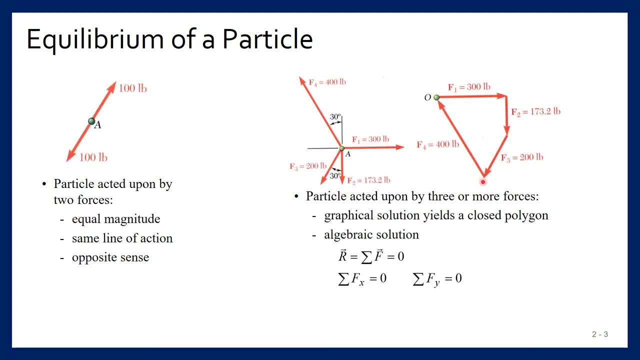 keep on making the other forces and then you will end up at the starting point. Another method which you can use is the algebraic solution. It is a summation of all the forces will be zero and in that case the summation of the forces in the x direction should. 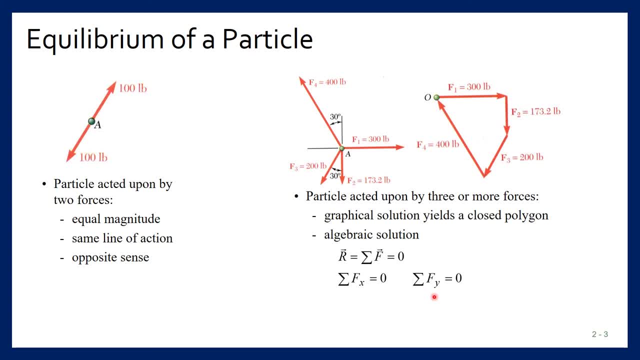 be zero, as well as the summation of forces in the y direction should be zero, and if you are applying the equilibrium in 3D, your summation of Fz should also be zero. That is, in case of 3D of fz should also be 0.. So this is all about equilibrium. Equilibrium is very, very important.